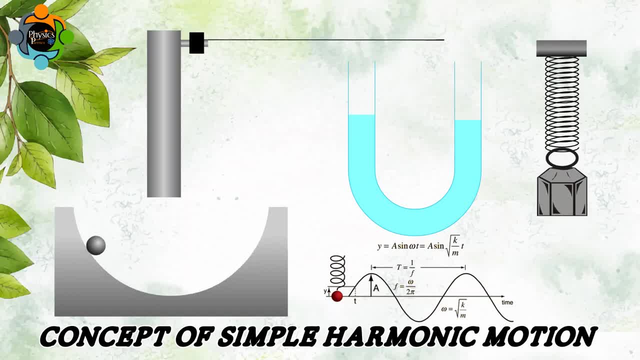 the concept. whenever we push and pull a system out of its equilibrium position and release it, it returns back to its initial position. This is how Ball nach dissipates. This leads to the oscillation we see in various systems around us, such as waves, springs and pendulums. 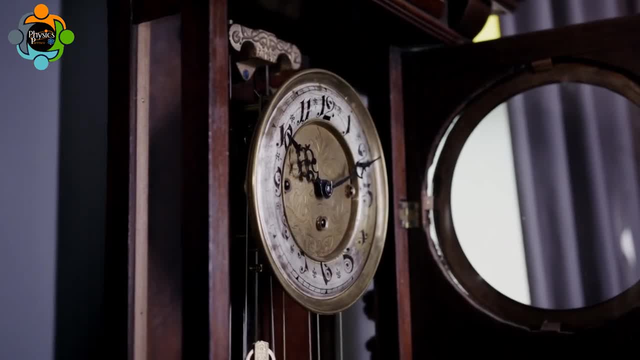 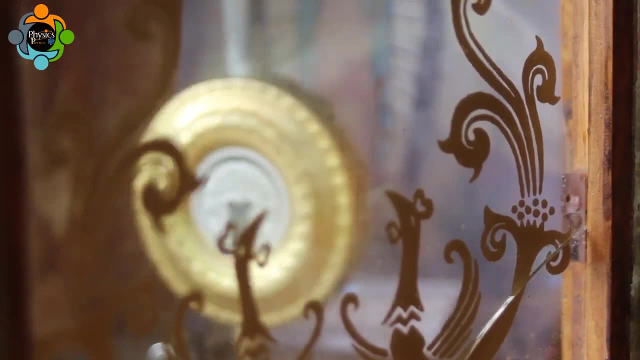 A real-life example of simple harmonic motion is the movement of a grandfather clock. The weight of the clock causes the pendulum to swing. This is how this şekl Irma- so called movement of the clock causes the pendulum to swing back and forth at the constant frequency, maintaining balance in the system. let's 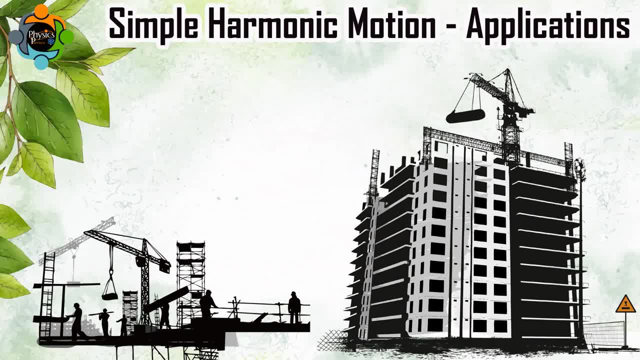 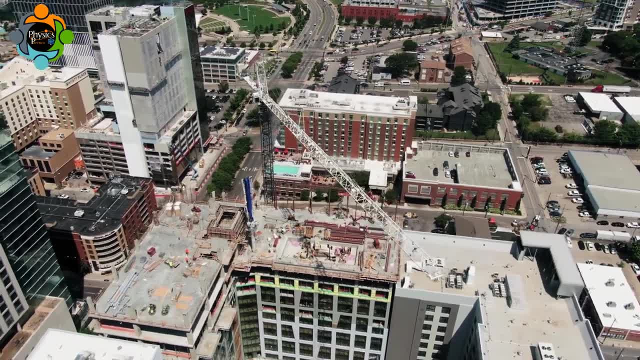 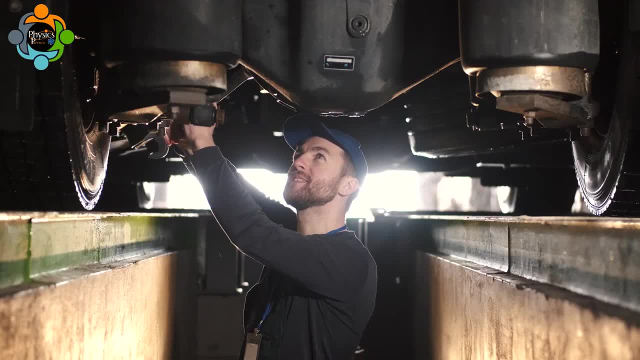 talk about the application of simple harmonic motion. simple harmonic motion find its application in various fields of science and engineering. the concept of oscillation is widely used in building structures to minimize the impact of the earthquakes or other natural disasters. the concept is used in building suspension systems in vehicles such as cars, bikes and trains to provide 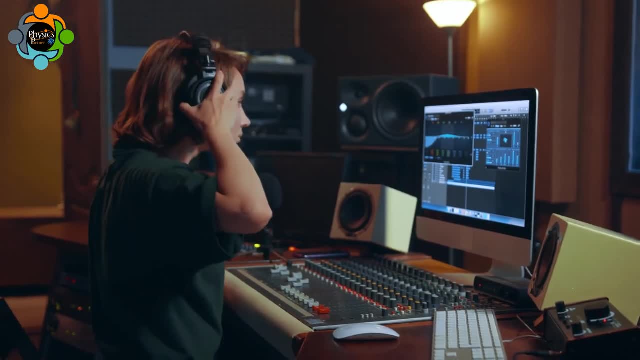 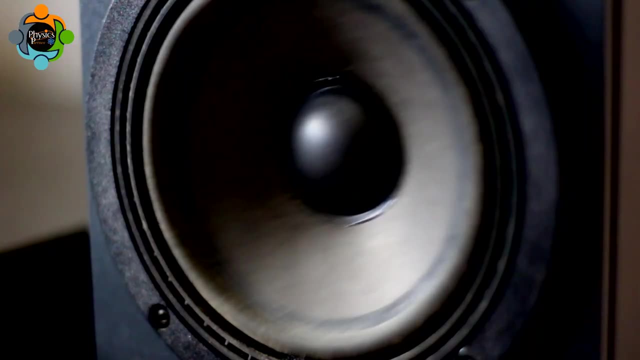 a smooth ride. in addition, simple harmonic motion plays a crucial role in the functioning of various electronic devices, such as the speakers, earphones and microphones, where the diaphragm or the speaker cone oscillates back and forth to produce sound. a very interesting example of simple harmonic. 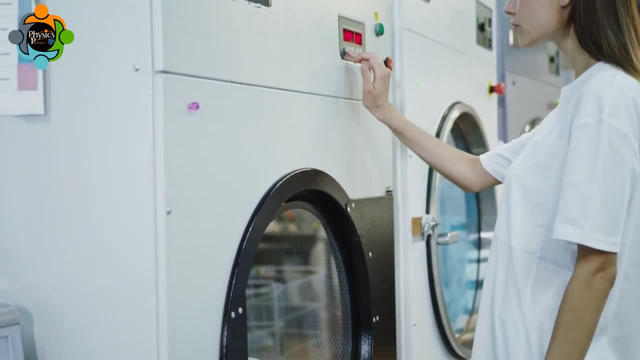 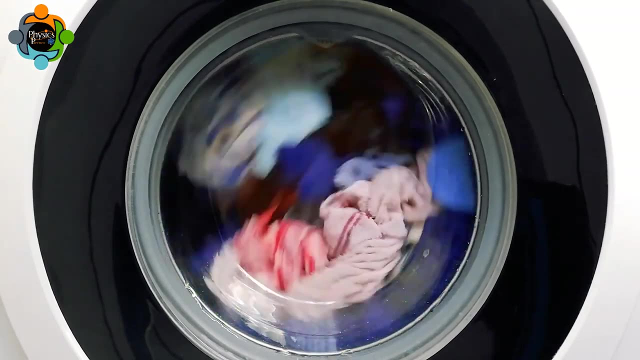 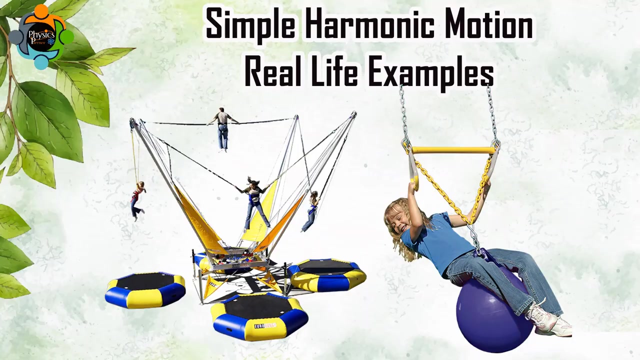 motion can be seen in the operation of a washing machine. the drum of the washing machine is made to oscillate back and forth in a sinusodial pattern, where causes the clothes to move around and get cleaned. the balance of the system ensures that the clothes does not damage due to vigorous movement. let's talk. 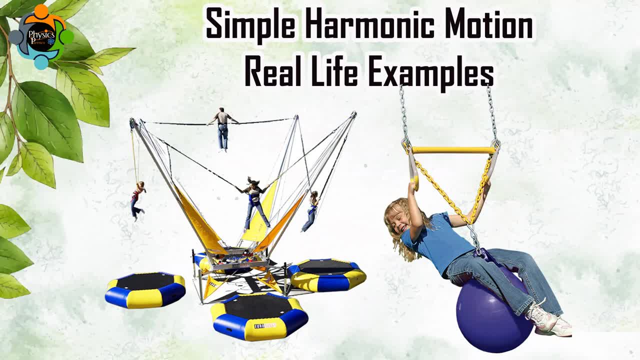 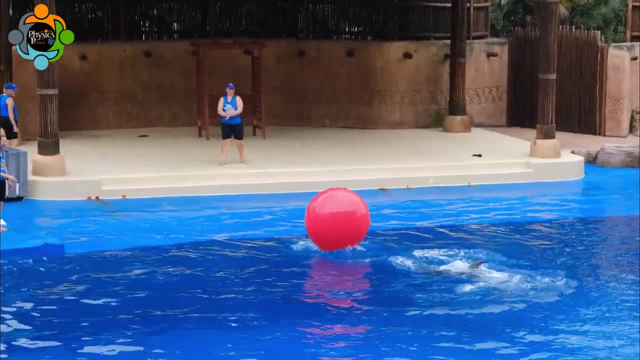 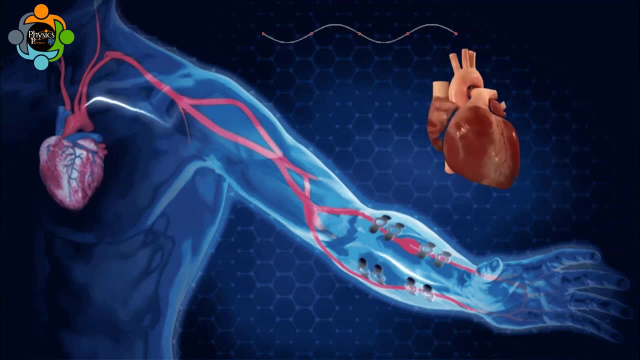 about the real-life examples. simple harmonic motion can be seen in various other daily activities. the movement of the swings or even the bouncing of balls can be attributed to the concept of simple harmonic motion. the motion of the human heart can also be explained using simple harmonic motion, where the heart 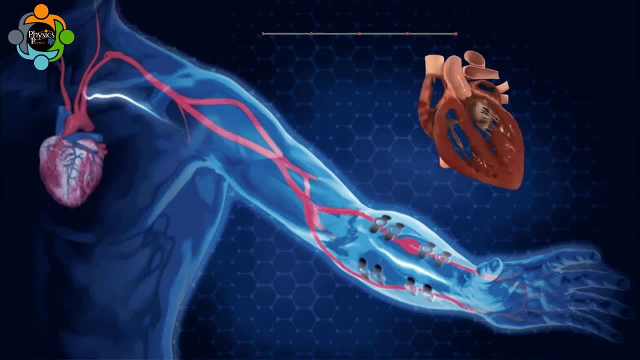 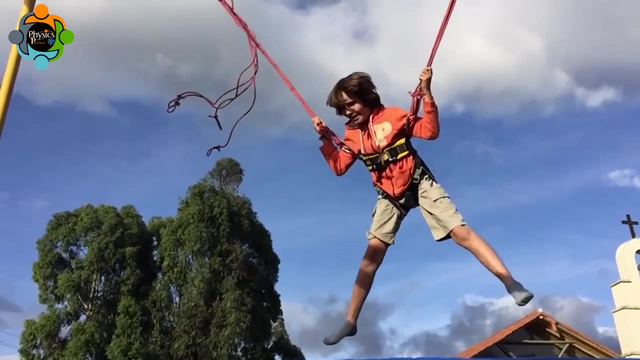 chambers follow a sinusoidal pattern to pump blood through the body. in conclusion, I have to say that simple, harmonic motion is an interesting concept that is found all around us, from the movement of the pendulum clocks to the bouncing of balls, the application and real-life examples of simple